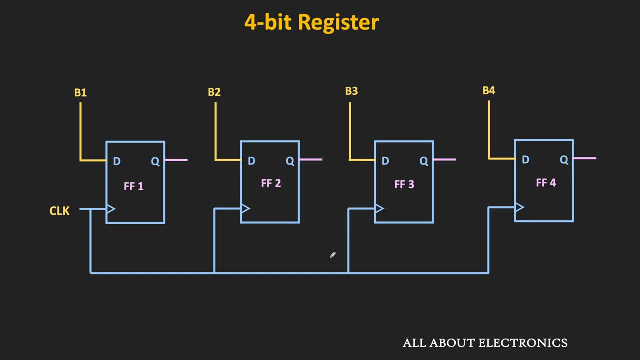 But practically this register is of no use. So let me explain why. Now, typically, if you see any synchronous digital system, then it has the master clock which is common between the different digital blocks. So let's say this resistor is also getting the common master clock. 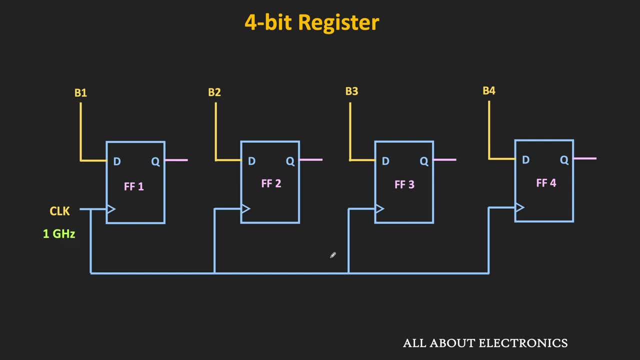 And let's say it is operating at the 1 GHz. That means the duration of the clock is equal to 1 nanosecond. So we can say that at every 1 nanosecond, whatever data is present at these 4 inputs. 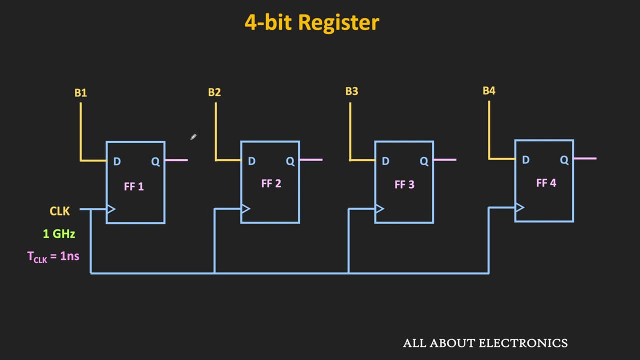 the same will be loaded into the resistor. So let's say we have some data which we want to store for the 300 microseconds. So here we also need to make sure that these 4 inputs, or the inputs of the data bus, it's 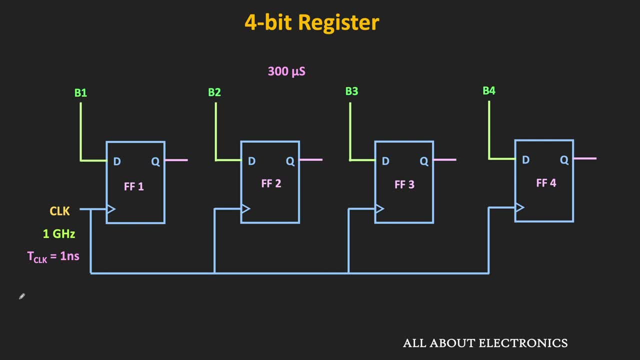 not changing up to 300 microseconds Because if the data changes before that time, then whatever random input is present at the data bus that will be stored in the resistor. That means we need to ensure that the data is available on the data bus up to 300 microseconds. 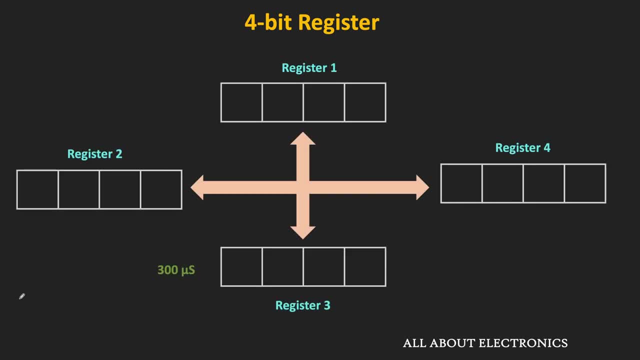 So in a way, here we are also occupying this data bus up to 300 microseconds And in between, If any other resistor in the system wants to access this data bus, then it won't be able to access that data bus. So let's see what we can do to avoid all these issues. 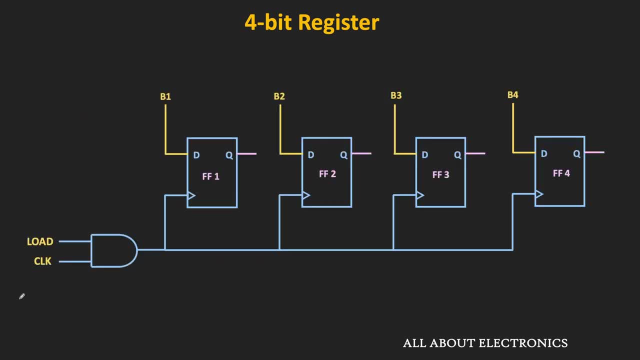 So the one solution is we can just enable the clock whenever we want to load the data in the resistor. So for that we can apply this clock to the resistor through this AND gate. So whenever this load signal is high, then only this clock will be delivered to the resistor. 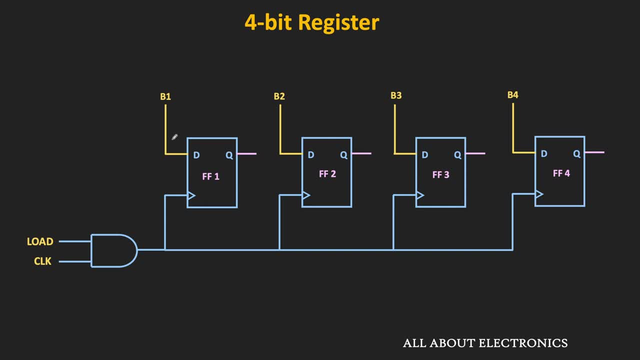 And whatever data is present at the resistor, it will be stored in the resistor, And whatever data is present at the inputs, the same will be loaded into the resistor. So whenever this load signal will become low, then this clock will also get disabled. 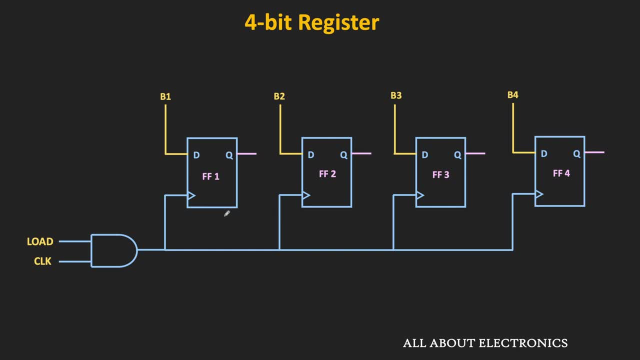 And, as you know, whenever there is no clock pulse, then the flip-flop will retain its current state. So, in this way, whatever data which is loaded into the resistor, it will remain as it is And, once again, it will change whenever this load signal is high. 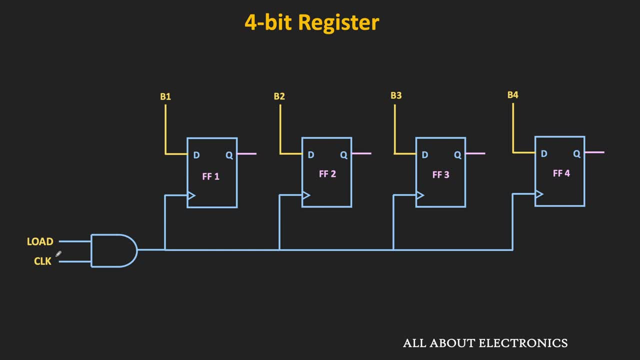 So in this way we are not occupying the data bus over the entire time, But generally this approach is not preferred And typically anything which controls the clock signal is usually avoided in the synchronous digital systems, Because here, due to this AND gate, this resistor will receive the clock after the certain propagation. 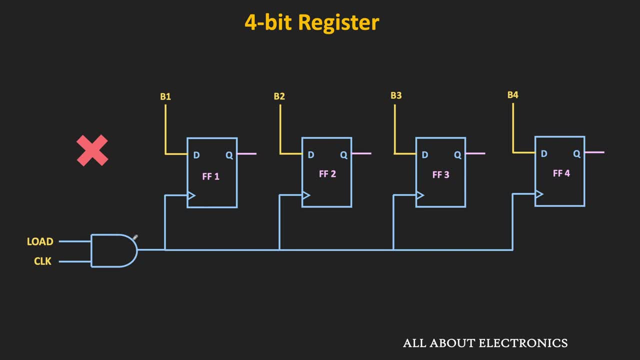 delay. That means there is a propagation delay between the master clock and the clock which is received by the resistor, And in the synchronous systems it is preferred that all the synchronous elements receive the clock at the same time. That means this approach is typically avoided in the synchronous systems. 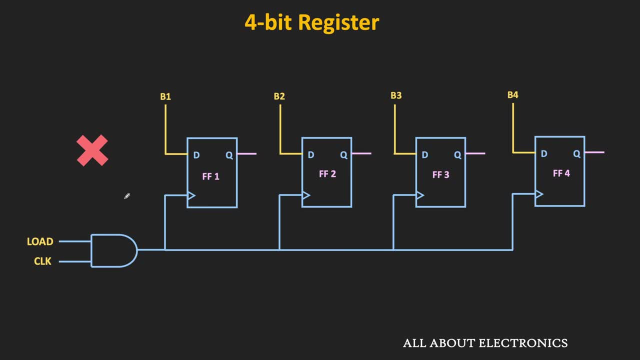 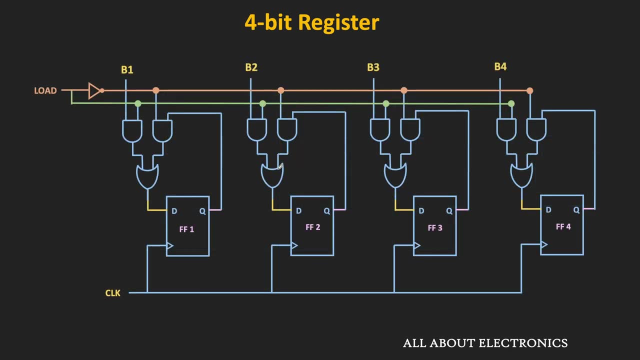 So, rather, controlling the clock signal, the operation of the resistor is controlled by the controlling the data inputs. So this is how the data bits are controlled using the load signal. So, as you can see, whenever this load signal is high, then the data bits B1,, B2,, B3 and 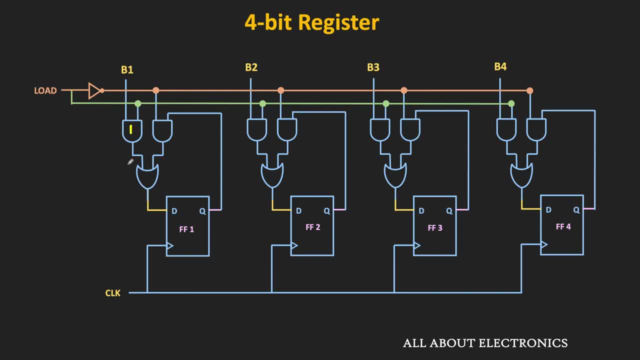 B4 will reach to the flip-flop through this AND gate And at the clock transition that data will be loaded. Now, whenever this load signal is high, then this load bar will become low And therefore the output of this second AND gate will become zero. 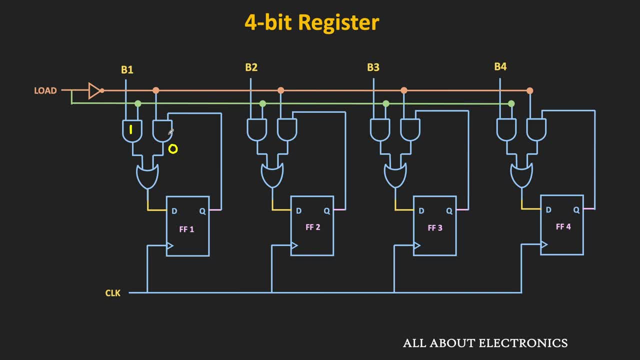 That means in that case, this second AND gate will remain disabled. Now, whenever this load signal will become low, then the output of this first AND gate will become zero. But now, since the load bar will become high, so this input will become high. 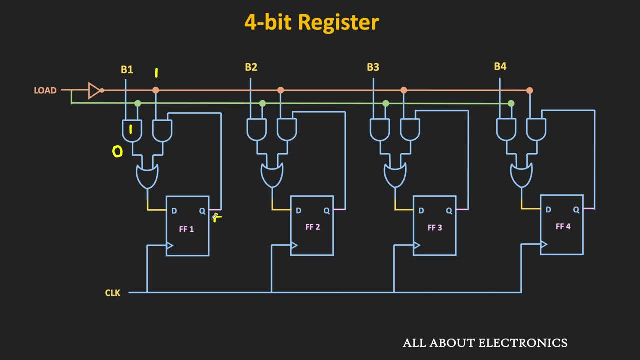 And now, whatever output is present at the top of the register, this input will become high And the output of the flip-flop the same, will be given back to the input And in this way, the flip-flop will hold its current data. 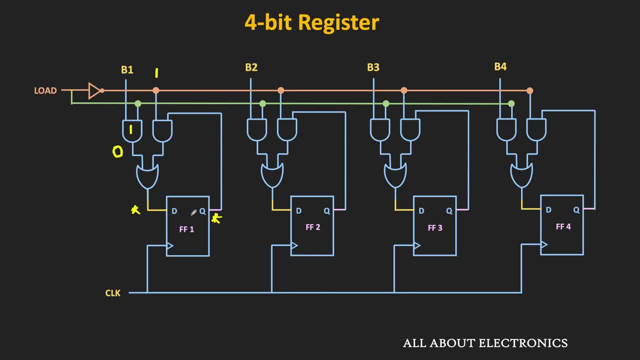 That means whenever you just want to load the new data, then first of all make the data available on this data bus And then after just enable this load signal, And when this load signal is low, then the register will maintain the previous data. 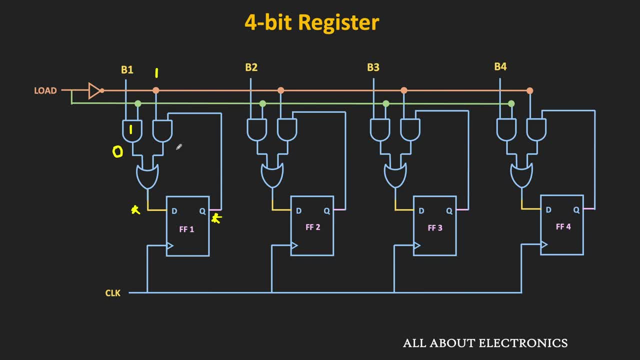 So this is the very basic register with the load input, And here Load signal is the synchronous input, Meaning that once this load signal is high, then the data will get loaded into the register only at the clock transition. So along with the load signal we can also have the asynchronous, clear input. 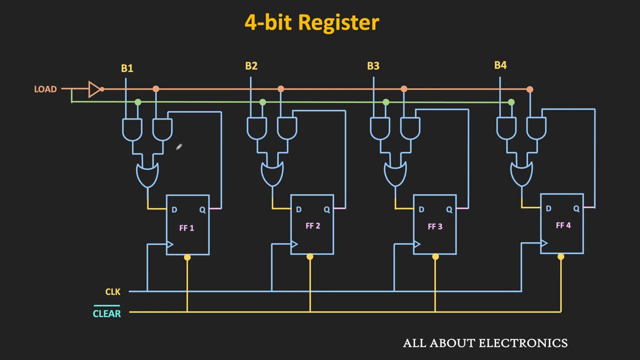 So here, as you can see, this clear input is the active low. That means whenever this clear input is low, then all the flip-flops in the register will get reset to zero. So if we represent the same circuit in the block diagram, 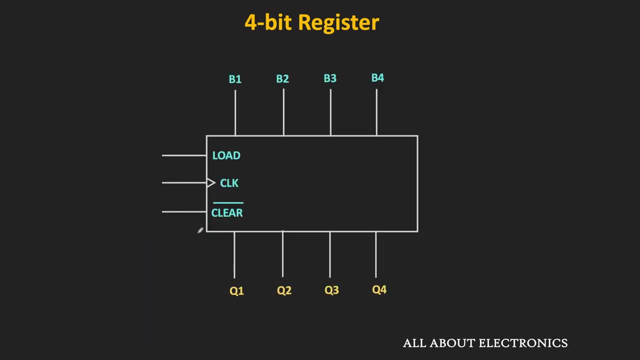 Then this is how it works. This is how it can be represented. So here this B1 to B4 are the inputs, while the Q1 to Q4 are the outputs, And apart from that we have also this load signal and the clear input. 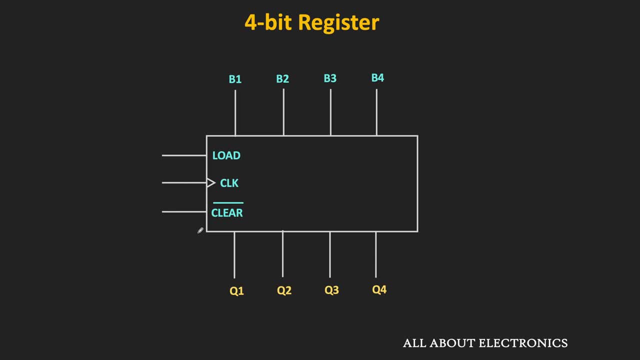 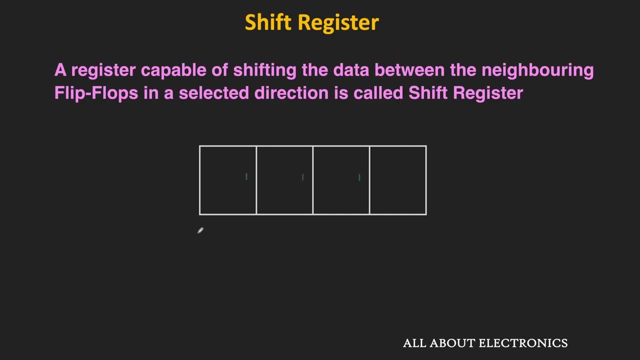 So in this type of register we can store the data or we can retrieve the data. But there is another type of register where it is possible to shift the binary data between the neighboring flip-flops of the register. So this type of register is known as the shift register. 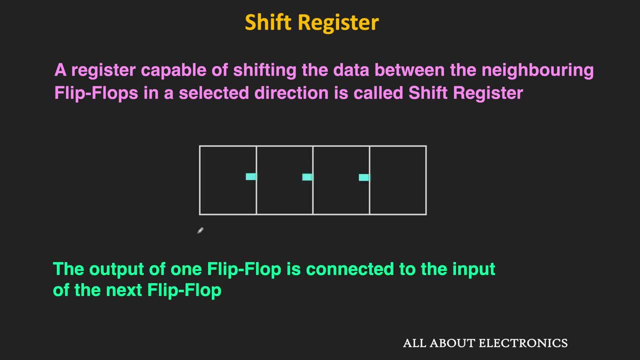 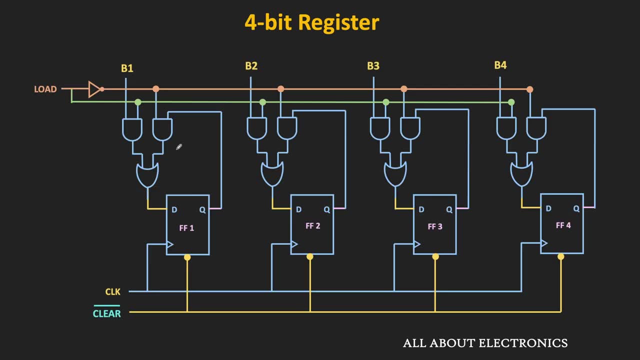 So in this type of register the output of the one flip-flop is connected to the input of the next flip-flop. So if you see the register circuit which I have discussed so far, in that there is no interconnection between the flip-flops, 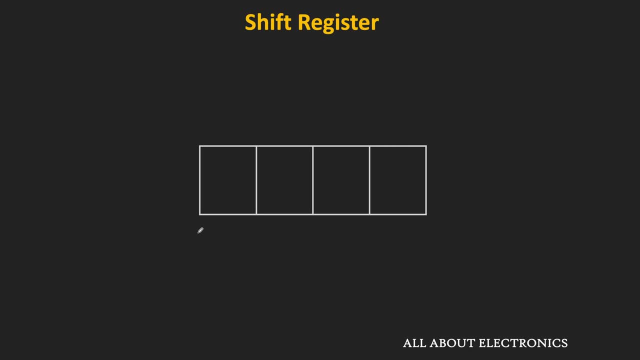 But in the shift register the neighboring flip-flops are the interconnected. So in this shift register there are two ways the data can be loaded. The one is the serially. That means at the every clock pulse The new bit will connect to the new bit. 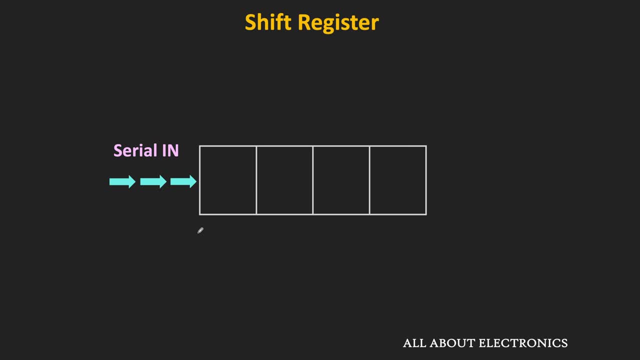 So in this type of register the output of the one flip-flop is connected to the input of the next flip-flop. So in this type of register the data will get loaded into the register. So if we have a 4-bit register then in the 4 clock pulses the data will get loaded into. 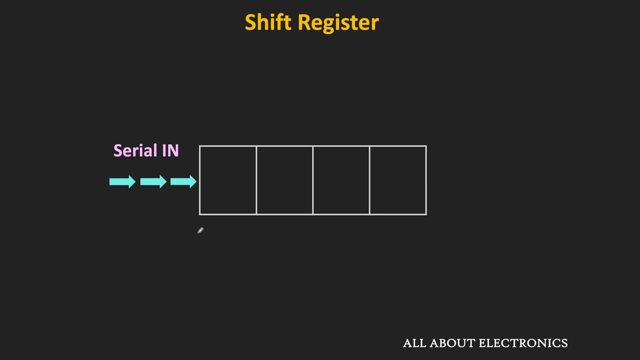 the register. So in this type of register the register has only one input. Now the second method of loading is the parallel load. So in the parallel load all the bits of the register will get loaded in the single clock. So if we have a 4-bit shift register, then for the parallel load this 4 input should. 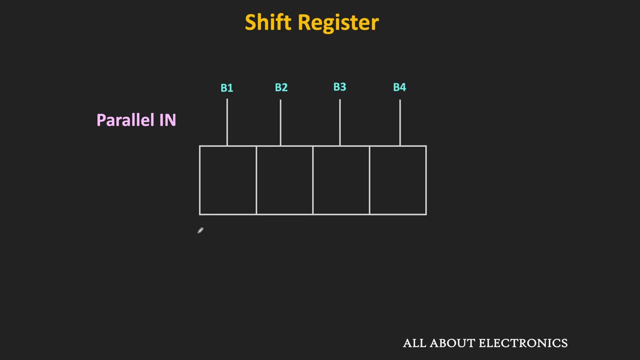 be accessible And by applying the inputs to these 4 lines, the new data can be loaded into the register in the single clock. That means there are two possible ways to load the data into the register. Similarly, there are two ways to retrieve the data from the shift register. 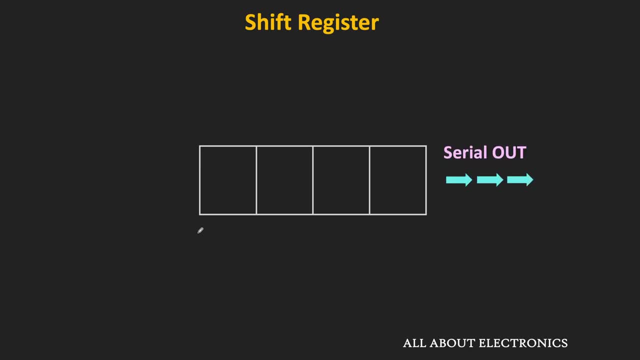 And the one is the serial out. So in the serial out we have only one output line And at every clock we can access only one output bit. So in a four-bit shift register To retrieve the data of the register we will require 4 clock signals. 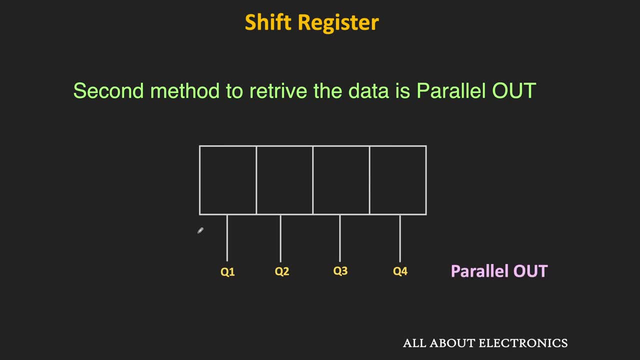 Now the second method is the parallel out. So in this parallel out we can access all the output bits in the single clock. So if we have a 4-bit shift register, then for the parallel out all the 4 outputs of the shift clock should be accessible. 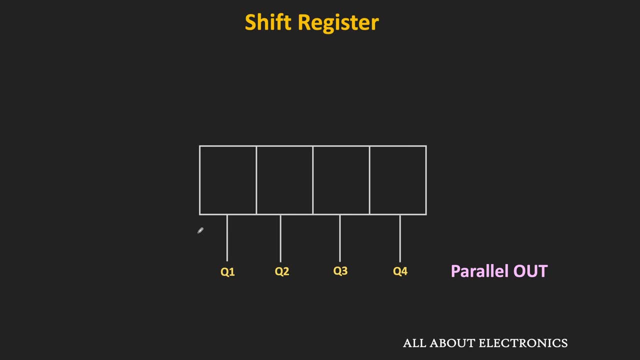 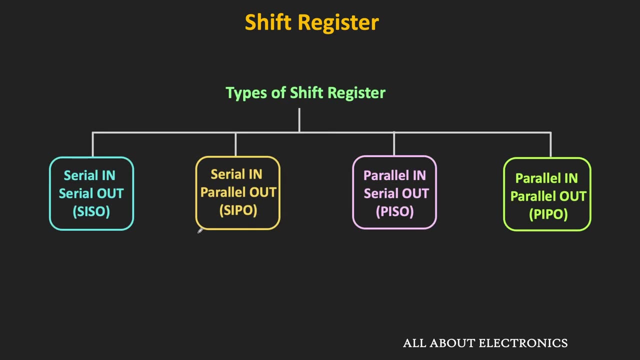 So, depending on how the data is loaded into the shift register and how the data is retrieved, we have total 4 types of shift registers, That is, Serial In Serial Out, Serial In Parallel Out, Parallel In Serial Out and Parallel In Parallel Out. So in the first type of register, 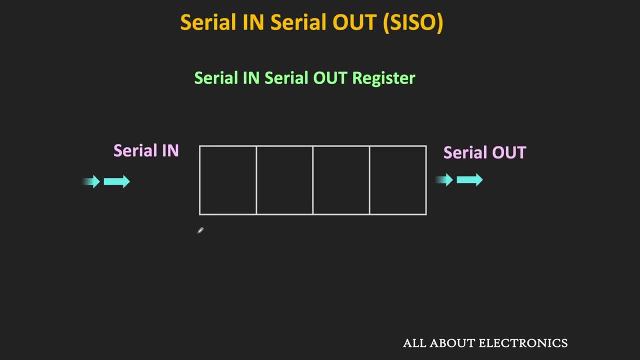 the data is serially loaded into the register and it is also taken out serially. Then in this Serial In Parallel Out type of shift register the data is loaded serially But it can be accessed parallelly. Then in this Parallel In Serial Out type, 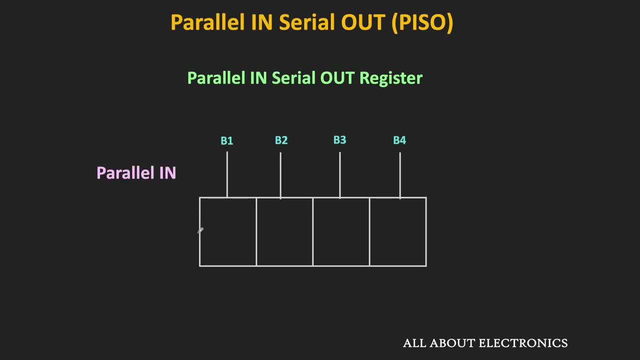 of shift register. the data is loaded parallelly but it can be taken out serially. And likewise, in this parallel in parallel out type of shift register, the data is loaded parallelly and it is also taken out parallelly. So this is similar to. 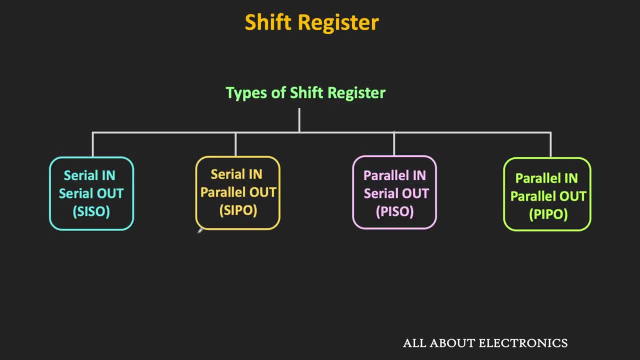 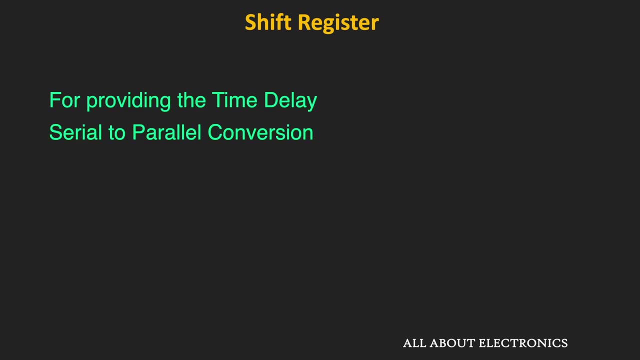 the register which we have discussed earlier. So these are the four types of shift registers. So, apart from the storage, because of its shifting property, these shift registers are also useful in many other applications, Like for the time delay generation and serial to parallel conversion. 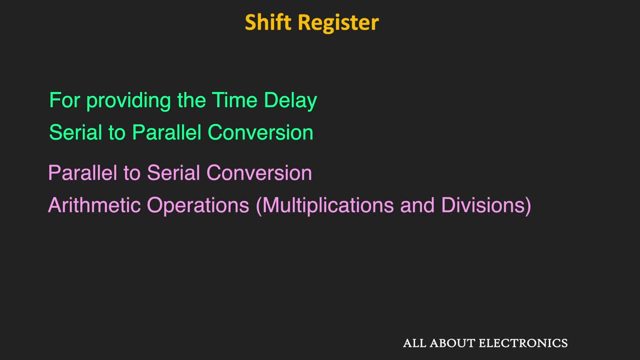 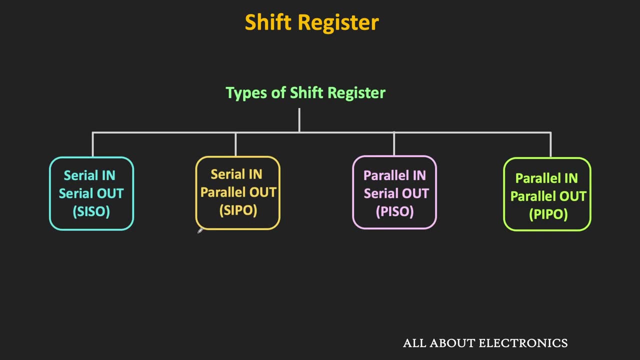 Apart from that, they can also be used for the parallel to serial data conversion, as well as in the arithmetic operations. So in the upcoming videos we will learn in detail about these different types of shift registers. But I hope in this video you got the basic idea about the. 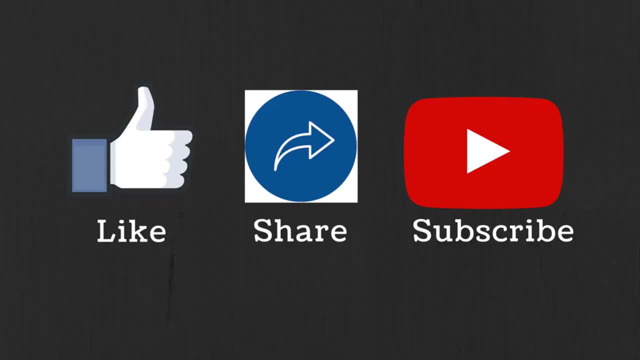 register and this shift register. So if you have any question or suggestion, then do let me know here in the comment section below. If you like this video, please hit the like button and share it with your friends. If you have any question or suggestion, then do let me know here in the comment section below. Hit the like button. 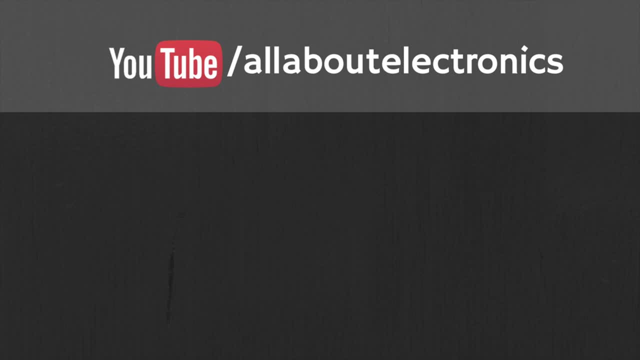 and subscribe to the channel for more such videos.